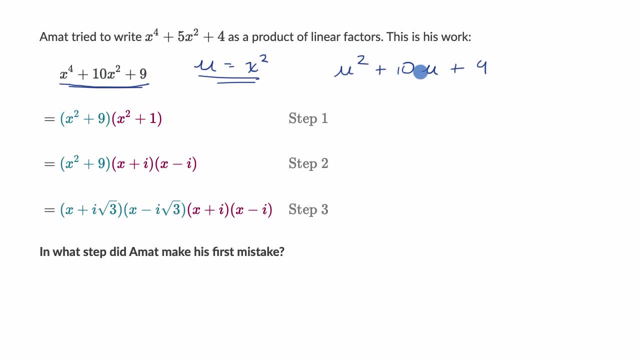 is so that you could write this higher order expression in terms of a second degree expression. And then we've learned how to factor things like this. many times We say: okay, what two numbers. when I add them, I get 10.. And when I multiply them, I get nine. 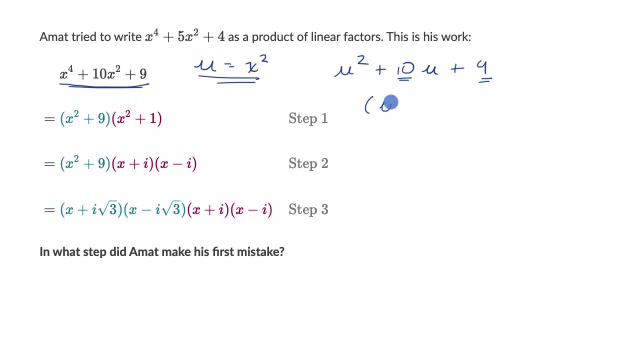 and it would be nine and one, And so you could write this as u plus nine times u plus one, And, of course, if u is equal to x squared, this would be x squared plus nine times x squared plus one, which is exactly what Amat has right over here. 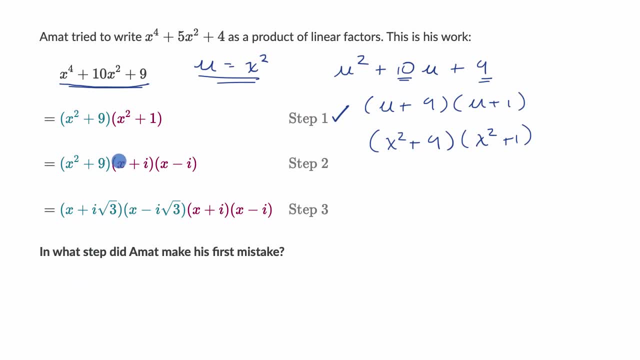 So step one is looking great. All right. now let's think about what Amat did in step two. They didn't do anything to x squared plus nine, but it looks like they tried to further factor x squared plus one, And this does seem right. 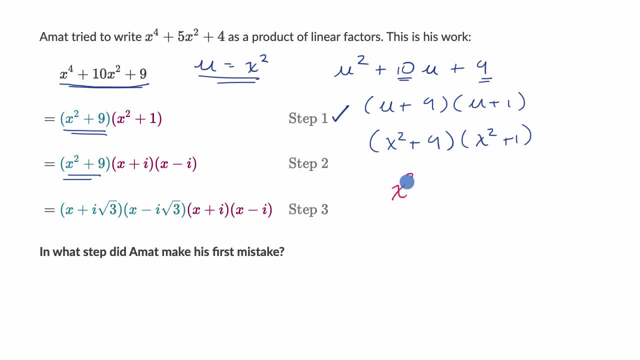 We just have to remind ourselves: just as you have a difference of squares if you're dealing with non-complex numbers, so we could rewrite this right over here as x plus a times x minus a, we could have a sum of squares if we're thinking about complex numbers. 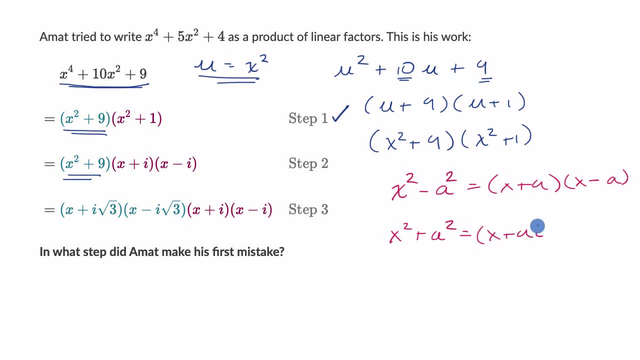 This is going to be x plus a i times x minus a i, And in this situation, well, the x is x and then our a would be one. So we're going to have x plus one i. x plus one i times x minus one i. 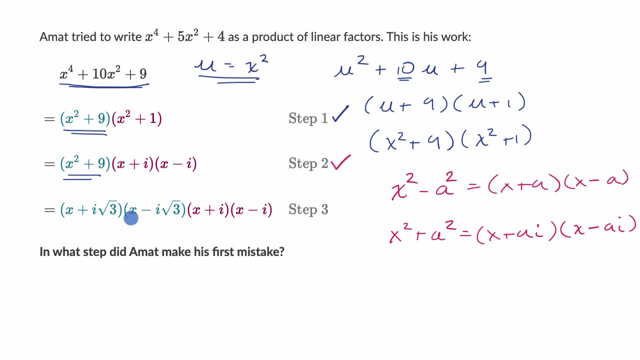 So step two is looking great, And now let's go to step three. So in step three, no change to this part of the of the expression, And it looks like Amat is trying to factor x squared plus nine, based on the same principle. 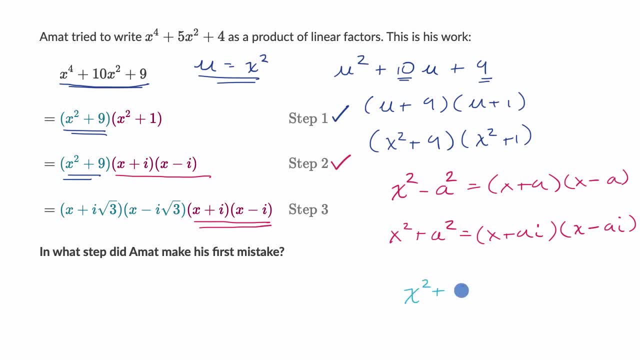 Now, x squared plus nine is the same thing as x squared plus three squared. So if you use this exact same idea here, if you factor it, it should be x plus three i times x minus three i. But what we see over here is: Amat took the square root. 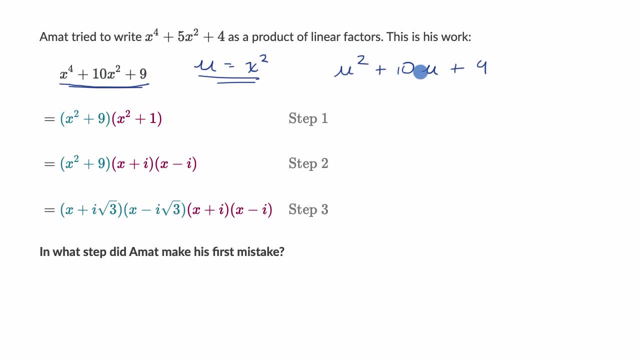 is so that you could write this higher order expression in terms of a second degree expression. And then we've learned how to factor things like this. many times We say: okay, what two numbers. when I add them, I get 10.. And when I multiply them, I get nine. 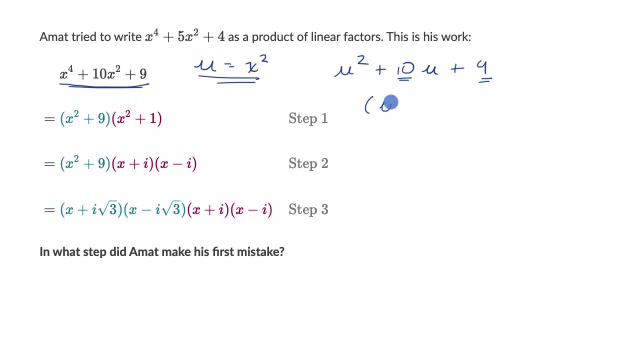 and it would be nine and one, And so you could write this as u plus nine times u plus one, And, of course, if u is equal to x squared, this would be x squared plus nine times x squared plus one, which is exactly what Amat has right over here. 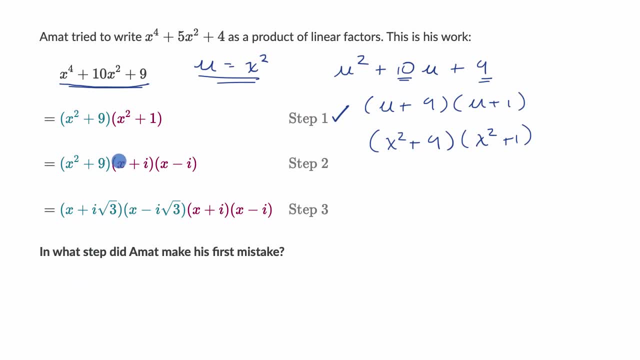 So step one is looking great. All right. now let's think about what Amat did in step two. They didn't do anything to x squared plus nine, but it looks like they tried to further factor x squared plus one, And this does seem right. 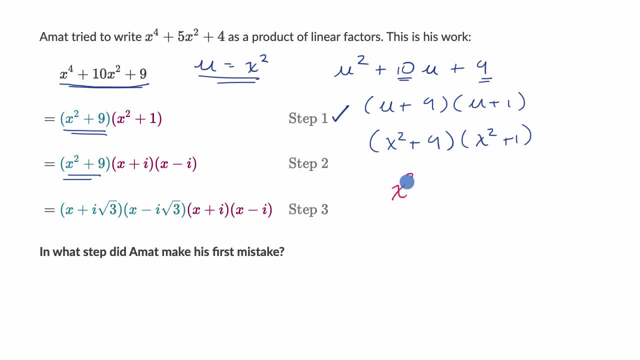 We just have to remind ourselves: just as you have a difference of squares if you're dealing with non-complex numbers, so we could rewrite this right over here as x plus a times x minus a, we could have a sum of squares if we're thinking about complex numbers. 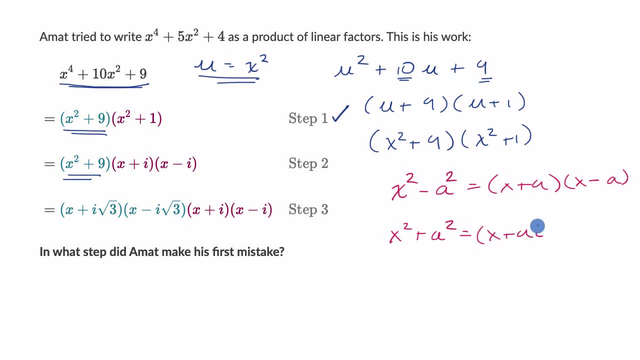 So this is going to be x plus a i times x minus a i, And in this situation, well, the x is x and then our a would be one. So we're going to have x plus one i, x plus one i times x minus one i. 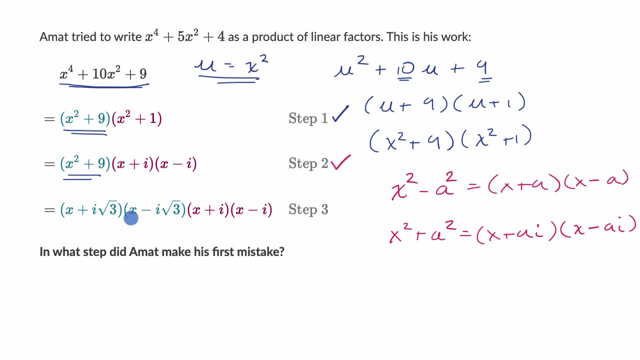 So step two is looking great, And now let's go to step three. So in step three, no change to this part of the of the expression, And it looks like Amat is trying to factor x squared plus nine, based on the same principle. 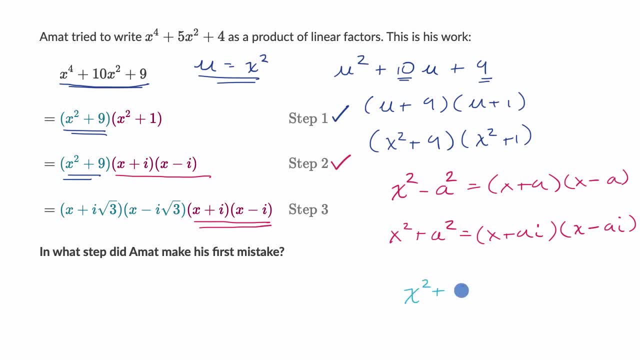 Now, x squared plus nine is the same thing as x squared plus three squared. So if you use this exact same idea here, if you factor it, it should be x plus three i times x minus three i. But what we see over here is: Amat took the square root.